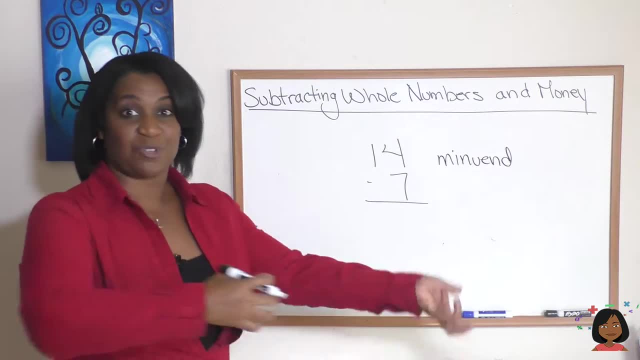 And the bottom number, the amount that we are subtracting from the minuend, is called the subtrahend. I know. 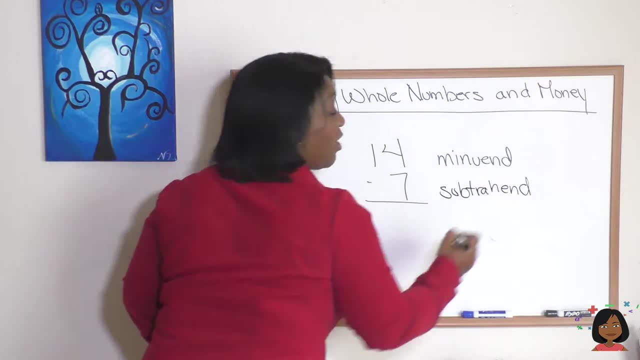 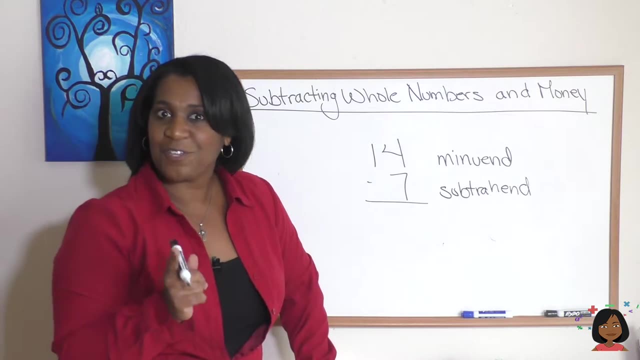 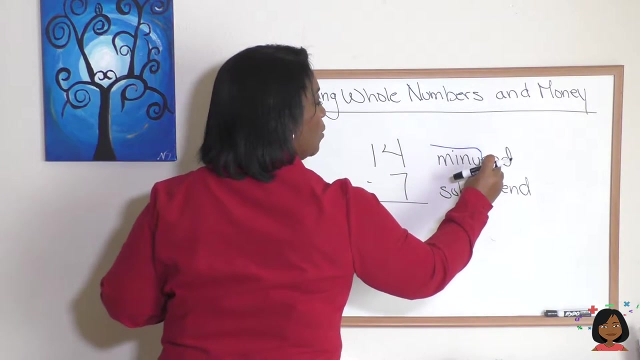 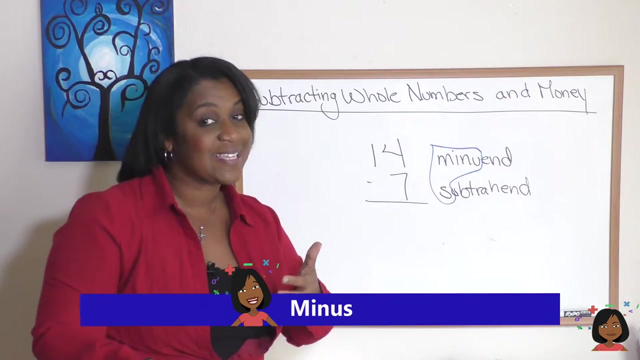 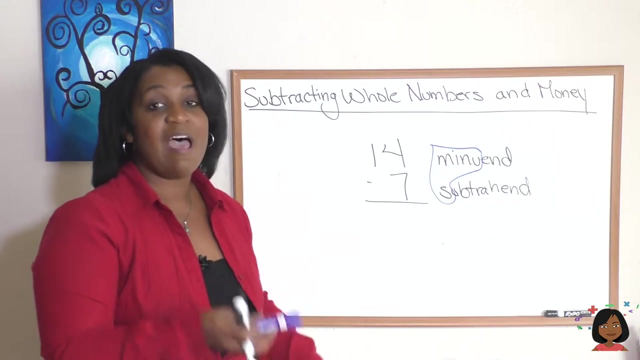 I was not really familiar with these terms for a long time in math, and I have a Nicole-ism for you, to help remember which one is which. If you look close, you might notice something. Minuend and subtrahend, if you pull certain letters out, it spells the word minus. And really, isn't that what subtraction is doing? We are minusing something? So, that will help you remember, the M has to always be the first one. Let's do it again, minuend, then subtrahend. And this will be important when we get to talking about missing numbers in subtraction. So, just remember that Nicole-ism. Let's keep it going. 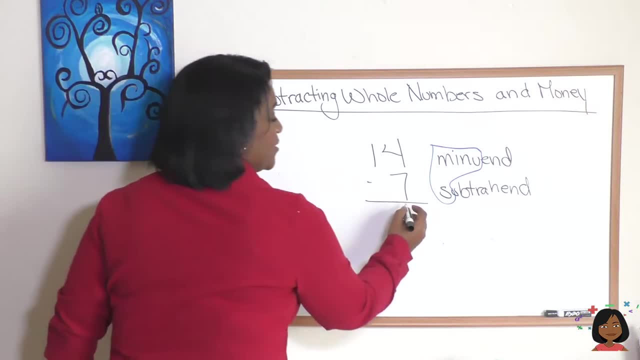 Let's do our subtraction. 14 minus 7 is 7. And this has a special name in math as well. It is called the difference. So there are your terms for subtraction. Let's keep going. Let's do subtraction. 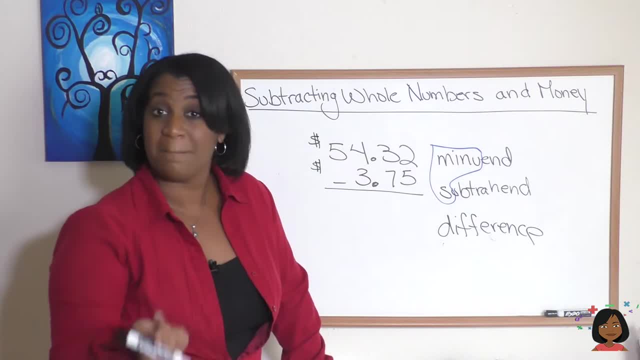 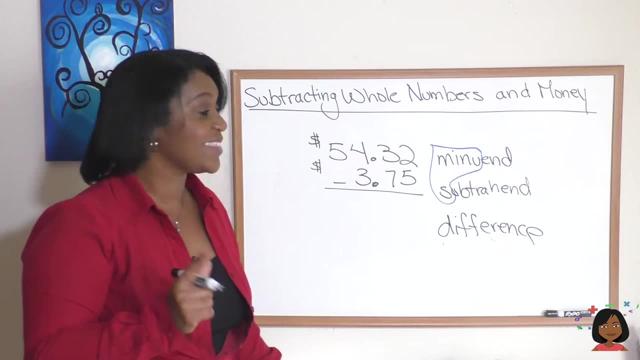 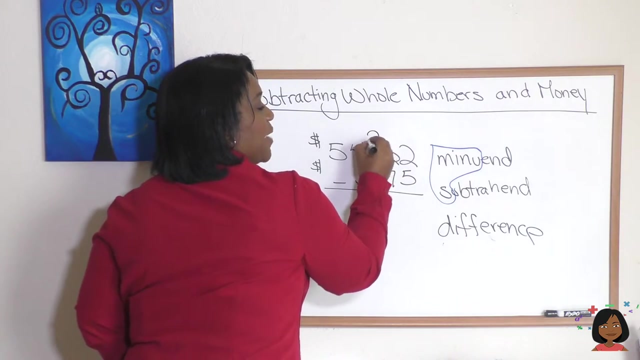 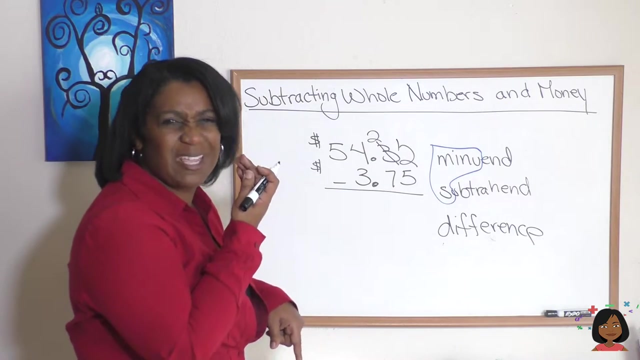 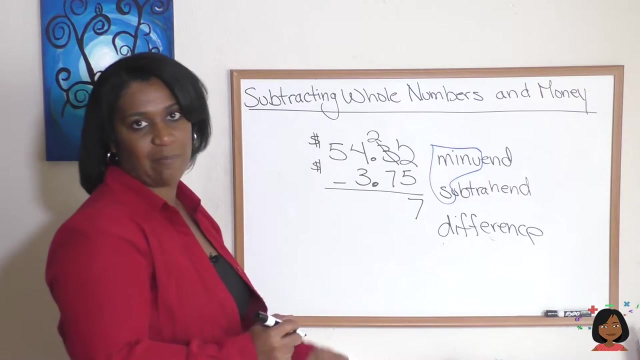 keep it going and this time do a subtraction problem with money there we have fifty four dollars and thirty two cents that's our menu end we've got three dollars and seventy five cents that's our subtrahent let's go ahead and subtract now you're going to notice right away we've got a bit of an issue can we do can we subtract five from two we don't seem to have enough so in math we do something called borrowing so i'm going to borrow technically 10 from my three across this three out make this a two and bring a one over to my twelve so i've borrowed ten because really this three is a thirty hmm here we go twelve minus five now we can do it is seven oh wait we have the same problem again don't we two minus seven can't do it so we're gonna borrow 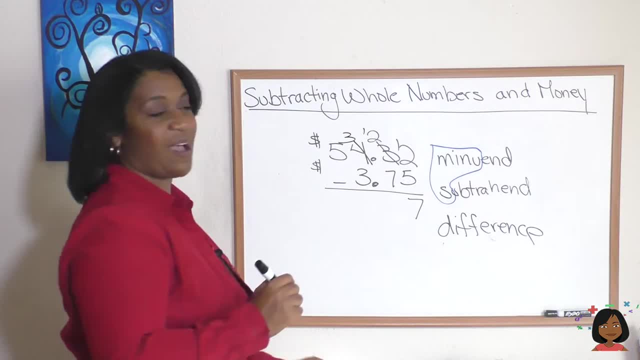 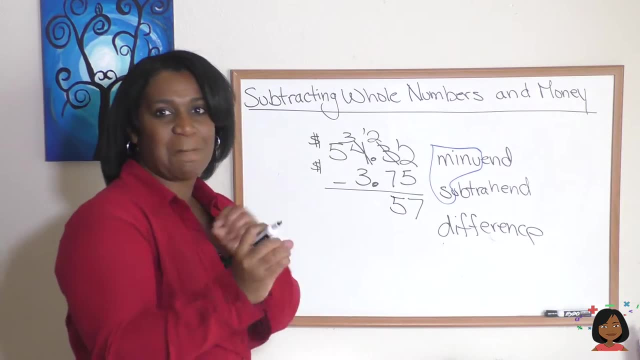 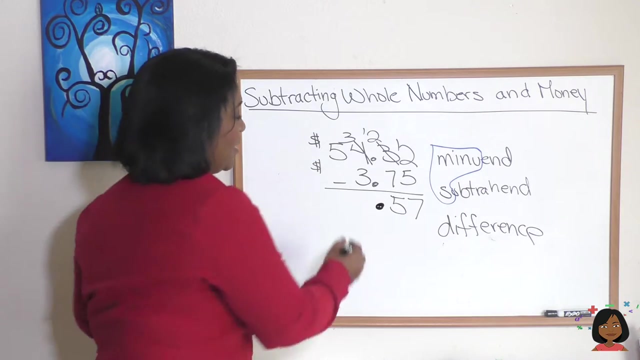 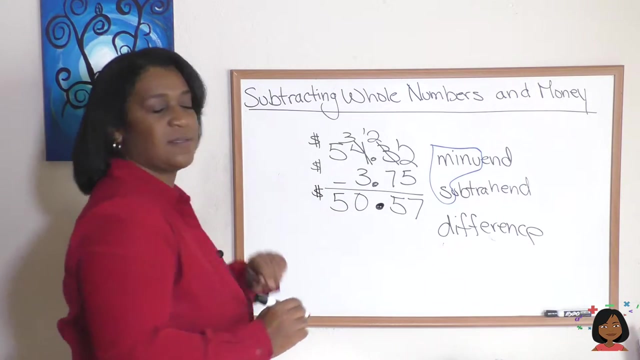 again and we're down to a three this goes to a twelve twelve minus seven this time is five and you know me i hit i hit my decimal point so i want to make sure that i don't forget them so i'm gonna go ahead and just write that decimal right now and keep it going three minus three is zero five minus there's nothing there so it's still five and i'm gonna add my dollar sign on we've got fifty dollars and fifty seven cents 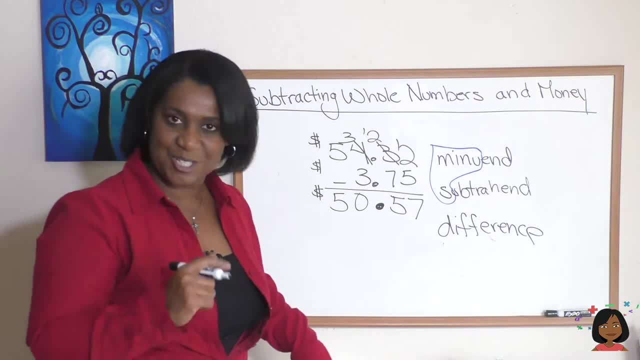 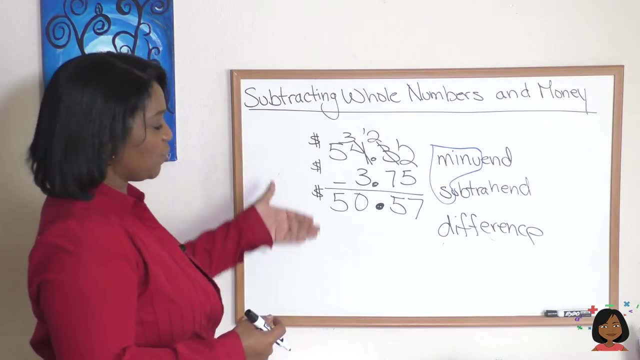 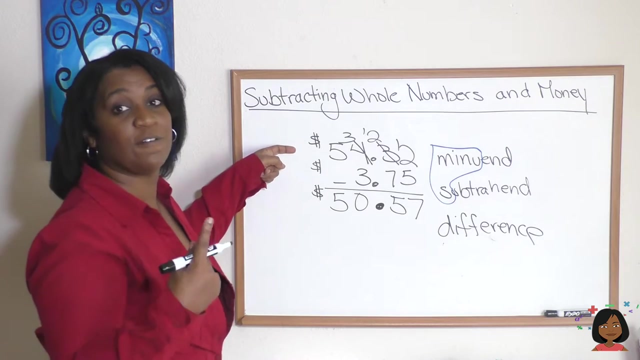 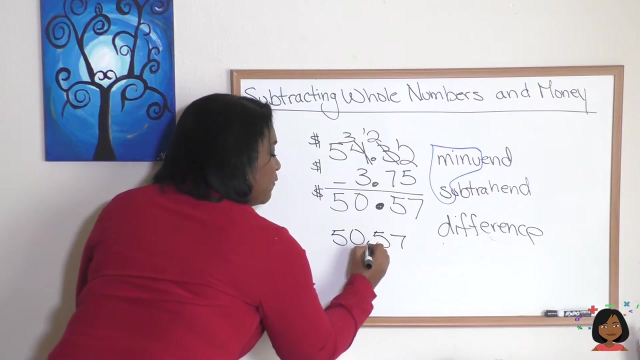 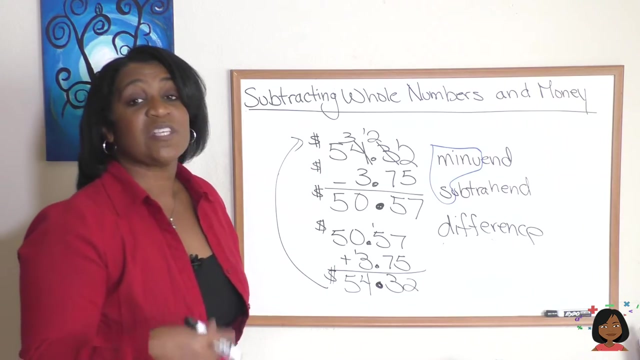 now i want to show you one of the cool parts about subtraction did you know that it has its own built-in answer checker yeah it does watch take a look at this so we subtracted but if i want to know that if my answer is correct i can do something called adding up if i start at the bottom 50.57 and i add 3.75 cents to it it should equal 54.32 let's see if it works i'm going to rewrite my problem down here 50 50 50 57 i'm going to add 3 and here we go 7 and 5 is 12 7 and 5 is 12 and 1 is 13 and there is my decimal so i don't forget it keep it going three and one is four and now we have our five don't forget our dollar sign and looky looky it adds back up so what we say is that subtraction undoes addition and addition undoes subtraction and that's how we have our built-in answer checker 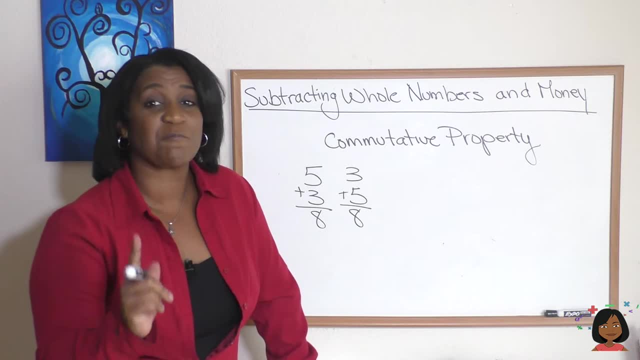 you might remember that for addition i talked to you about the commutative property of addition 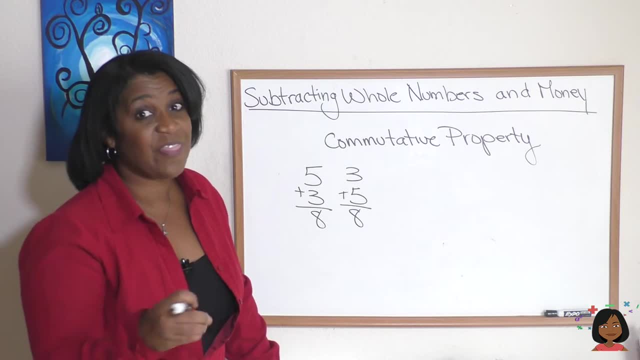 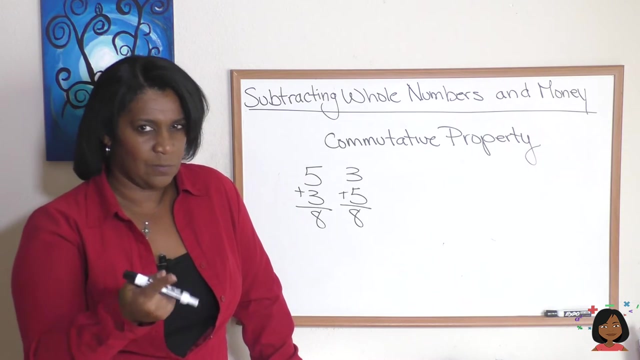 which tells us that it doesn't matter which order we add the add-ins in we'll still get the same sum right you might remember 5 plus 3 is 8 but 3 plus 5 is also 8. but let's check and see does this thing work for subtraction i don't know let's check it out let's say i had the number 11 minus 7 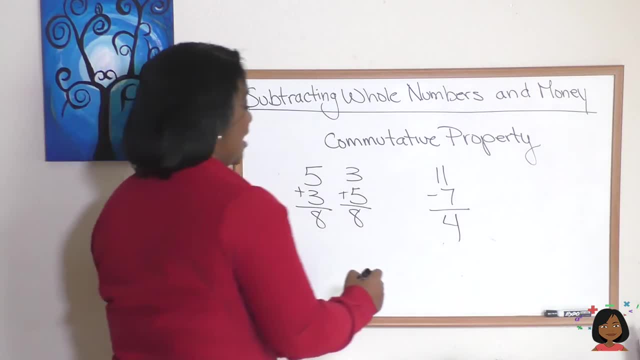 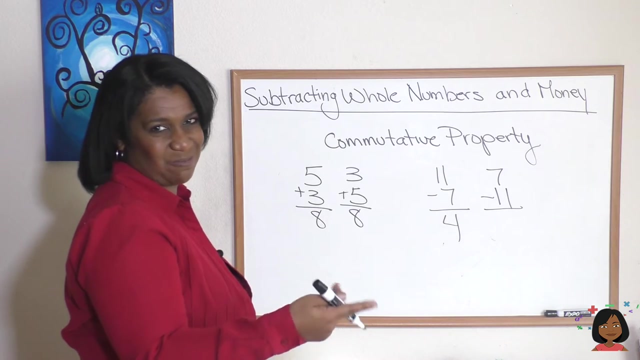 11 minus 7 is 4. let's try the same thing that we did here over here with subtraction so we're going to do 7 minus 11. well 7 minus 11 we're not going to get 4. we're actually going to get a negative number which is we're not talking about that right now so 7 minus 11 does not give us 4. 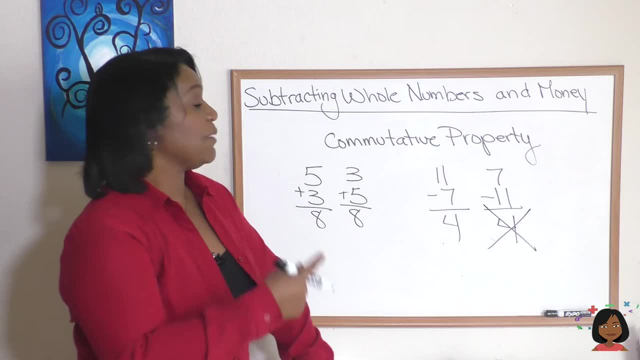 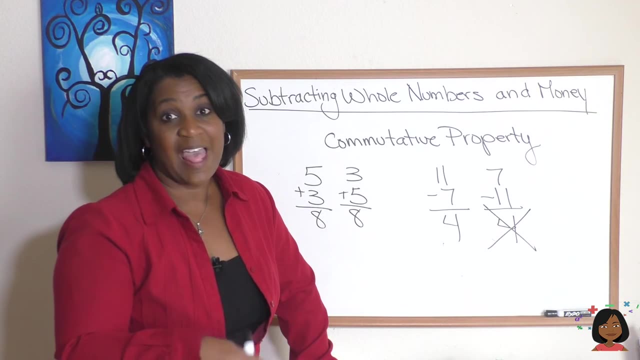 boom boom that's not correct so what does that mean it means that subtraction does not have a commutative property like addition does and that's it that's your quick review on subtracting whole numbers and money 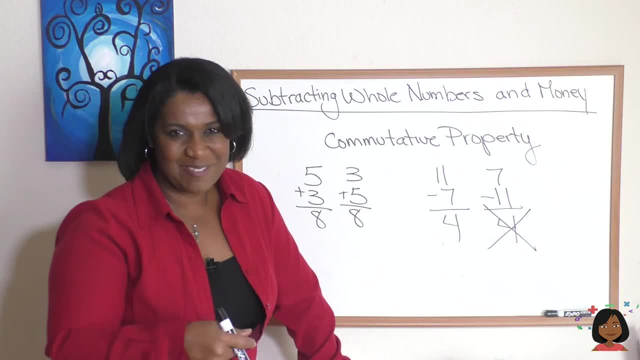 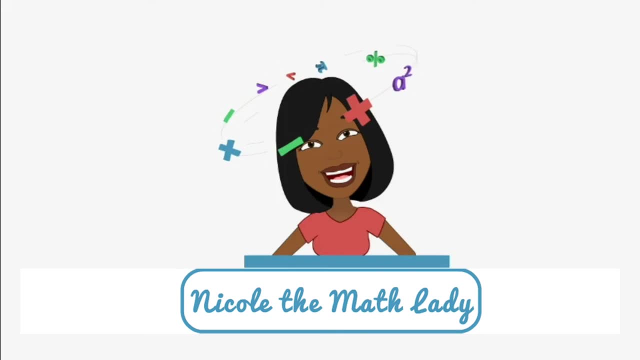 i hope that was easy for you i think so all right hope you're having a great day and i will talk to you next time bye